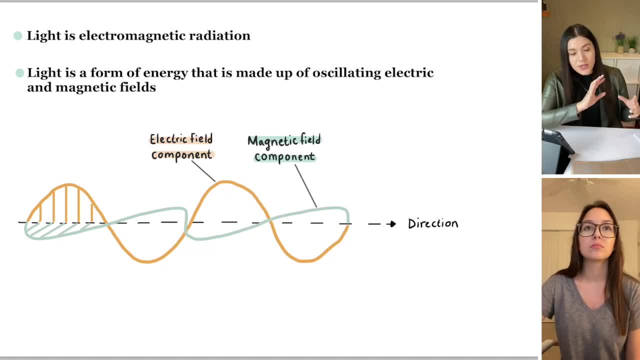 spectrum, And the main thing I want to do with this one is sure, we'll talk about the concepts and we'll talk about the different terms. that are typically multiple choice questions, But the main ones that I see students struggle with is just the calculations. So, because there are multiple, 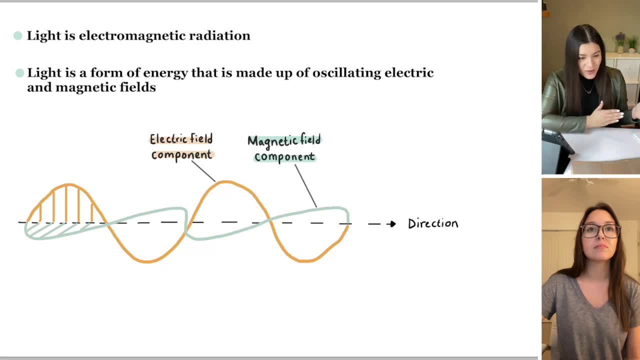 formulas that you might need to memorize or he might provide that. I'm not sure. typically they have you memorize it, unfortunately. Okay, But I really wanted to practice a lot with those because they tend to be kind of like it's just word problems, It's a bunch of words, Yeah. 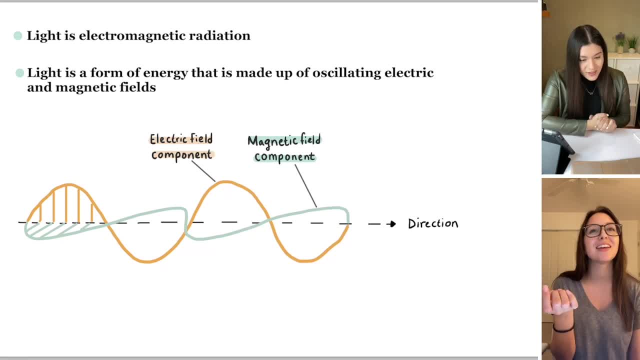 It's a bunch of word problems. So it's kind of like: Is this the Planck's constant thing? Because I think he said we do have to memorize that. Okay Yeah, Okay Yeah, Then. yeah, it's that. And then. 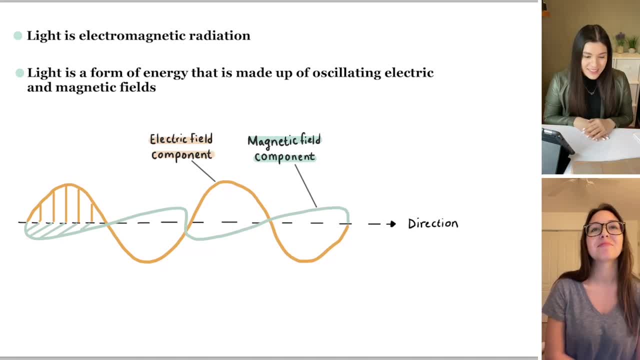 it's like the speed of light, like the C constant. Yeah, I think he said we need to know those. Yeah, Okay, Okay, Well, let's just. let's start off with just the concepts, understanding where everything comes from When we're talking about the electromagnetic spectrum. 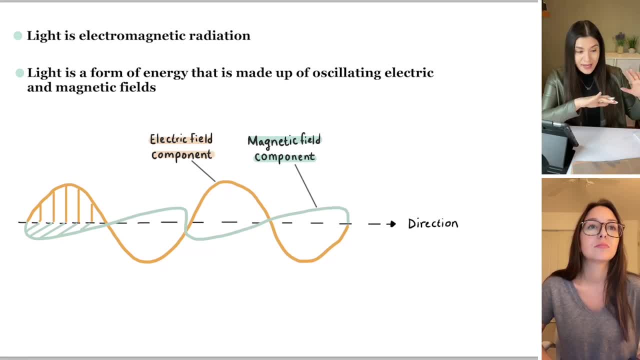 I kind of want to take a step back and look specifically at something known as the electro magnetic radiation. So all that is is light, Like all of these things that we're really talking about is a bunch of fancy words for just light. Okay, That's all we're observing here Now. 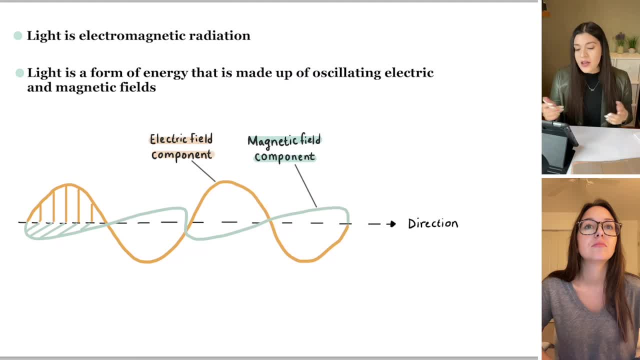 just to kind of know these definitions is going to be important. Just knowing that light is a form of radiation or electromagnetic radiation, All that means is that light is some sort of form of energy, And then the reason why we tend to see like light waves or those waves, 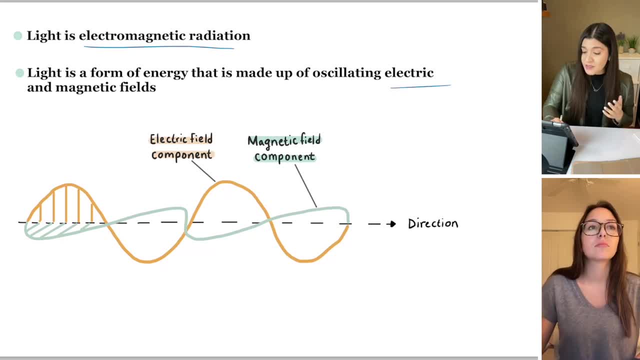 is because we have a different electromagnetic fields, So both electric and magnetic fields that are oscillating, just meaning they're moving back and forth. So we're literally going to get that kind of like wave form because they're just literally moving back and forth Like we're going. 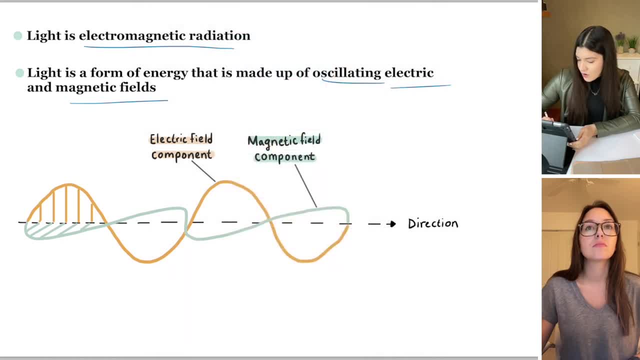 to see. let me highlight: we're going to see our electronic field up here and then it's going to come down Right And that's where we kind of like get that waves, that wave sort of formation. Let me put this in blue, and then same with the magnetic field. 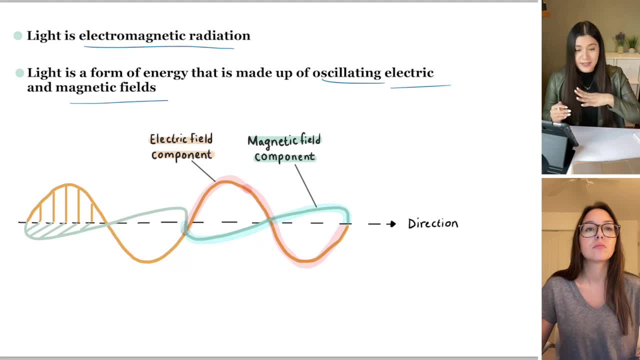 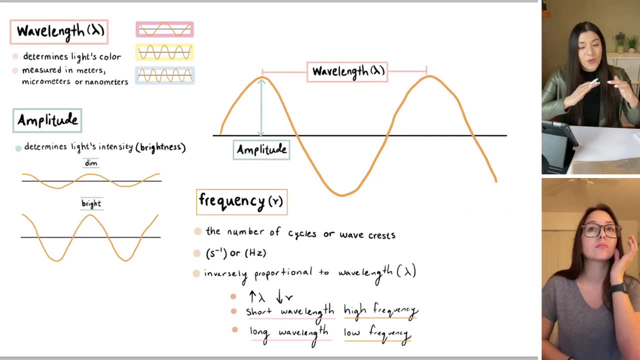 Okay. So it's really all just kind of like those waves. That's it. That's the main concept here that we're going to keep looking at, Okay, But we're going to get into into a little bit more detail understanding the different parts of a wave. So, the major things to know, I'd say these: 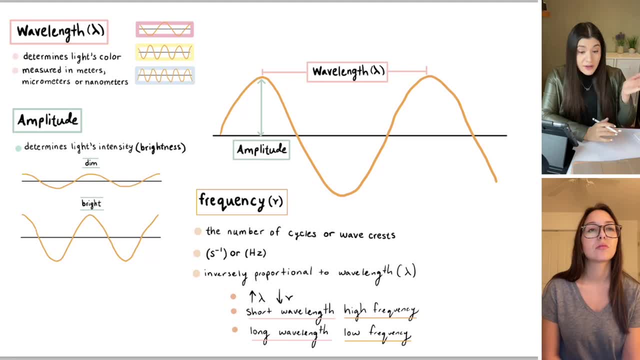 three is understanding um. one, how to calculate them and two, what they actually do. So we have a wavelength, and a wavelength is basically just telling us, um, what the color of the actual light is. So if we change the wavelength, we change the color. So, if you'll notice here, 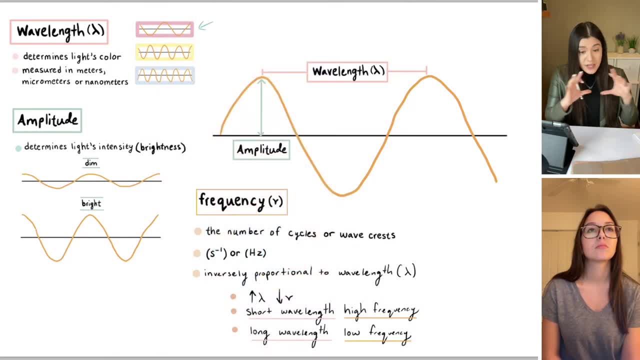 this top line. well, this is a little bit wider, I'd say a little bit more stretched out for that wave, And that tells us: okay, it's actually going to be red. If I were to kind of compress it a little bit more, it changes the color to yellow And then so on. If I compress this even, 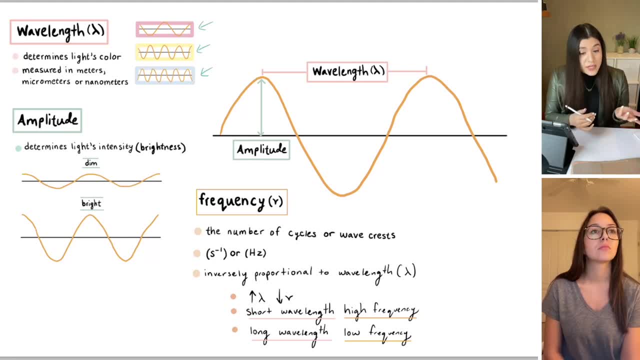 more. it changes it again to blue. uh, something to note here: for wavelength, the different units that you're going to see is meters, micrometers and nanometers. The most common one that most tests will actually have you put the answer in is going to be: 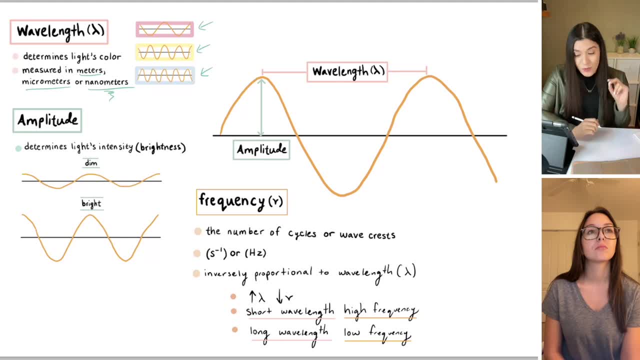 nanometers. So just a huge hint right there: that wavelength needs to typically be in nanometers, unless they specify that they want it in meters or something else. Next is the amplitude. So it's pretty much just talking about how high that wave would be, And then specifically it's going to. 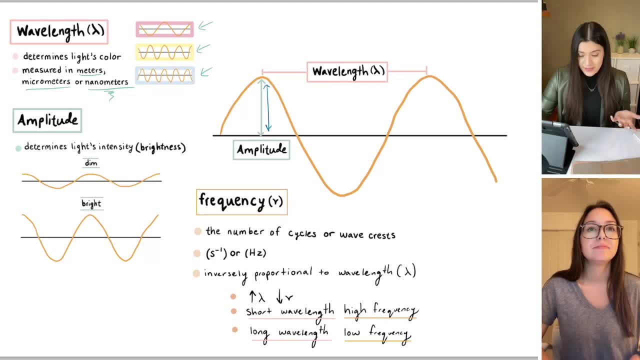 talk about the brightness of the light. So how intense is that light? So, once again, if I were to look at this one, this is completely stretched out. that wave is stretched out, then I know, okay, it's going to be more dim. If I were, 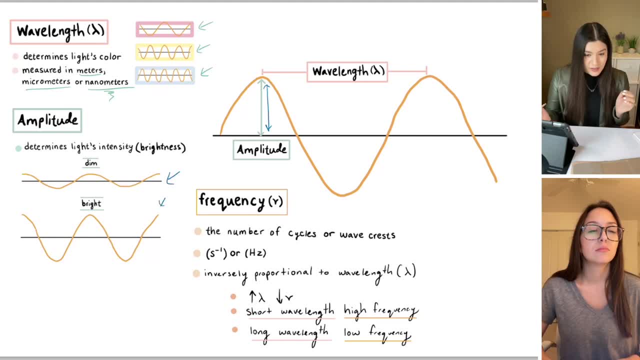 to kind of compress it a little bit more. it's going to be brighter, Okay. So understanding those like properties, and seeing what changes whenever we change the wavelength and the amplitude, those are multiple choice questions for you right there. Okay, Good to know. And then same with our. 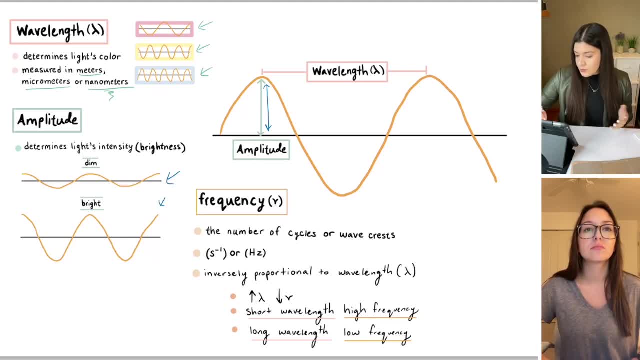 frequency, just understanding what that is. So our frequency, which is represented by kind of like this V looking shape, but it's not a V- There's going to be a little bit of a difference between the amplitude and the amplitude. So if I were to compress this a little bit more, it's going to be. 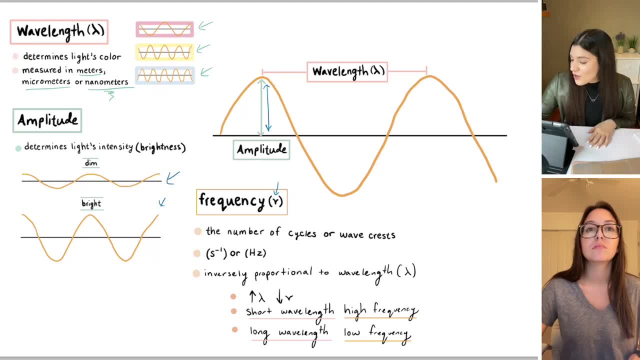 like a main differentiator right there We will talk about. so this is frequency, This V is velocity. Why did they choose that? I wish they didn't, but it's really similar, So be aware of that, Okay. And then our frequency is basically just the number of cycles that we have. So by 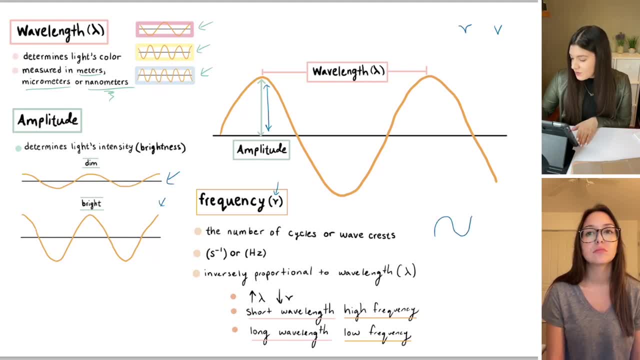 number of cycles. I mean like, oh okay, this is one cycle. If I were to continue, oh okay, that's another cycle. So, however many cycles we have, or wave crest- and I'll explain what that is in a 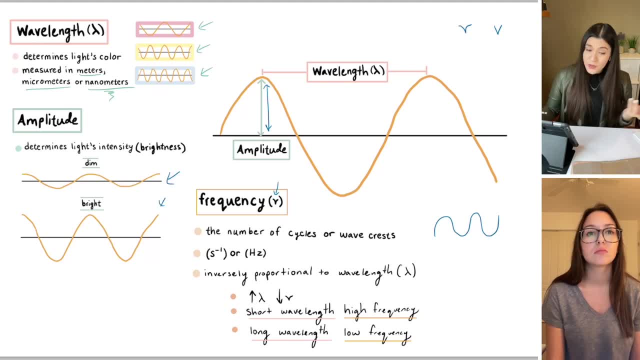 second. What else? to look at, the units. units are always important. So for frequency, you're either going to see that this is seconds to the negative first, or in Hertz. And then just something to definitely know is that one Hertz is equal to one second to the negative first. 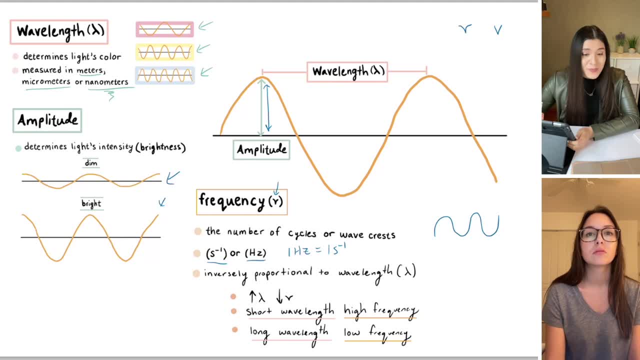 just in case they don't provide that. definitely know that, because it will come in handy with a lot of our calculations. Okay, And then the last thing on this slide is just talking about the relationship between, the relationship between frequency and wavelength, So understanding that they are inversely proportional. just to click. 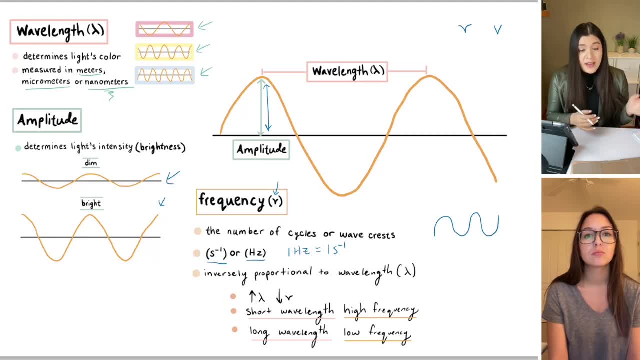 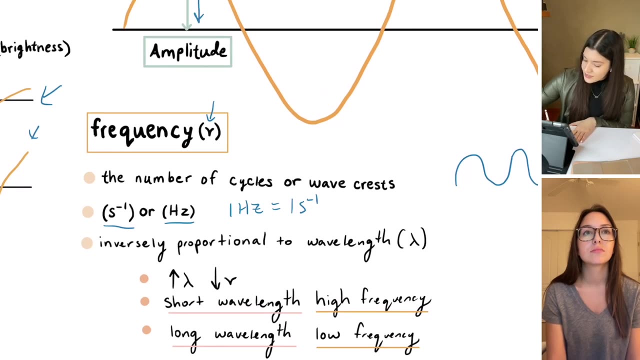 review on math. whenever something is proportional, that means as one increases, so does the other. whenever they're inversely proportional, that means one increase increases and the other one decreases. Okay, So looking at this one, that just means as we increase. 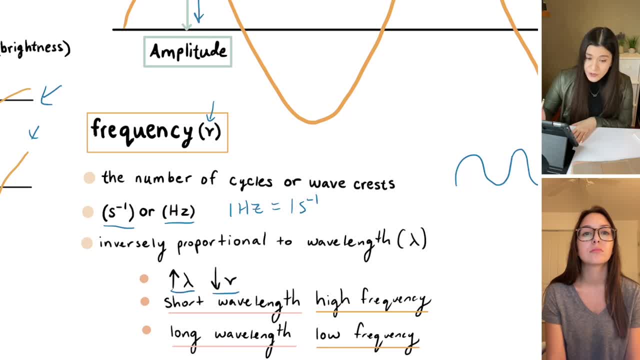 the wavelength number, then we're actually going to decrease the frequency. So let's kind of put that into understanding. So if this is a shorter wavelength, then we're going to have a higher frequency, and vice versa: If we have a longer wavelength, we're going to have a lower frequency. 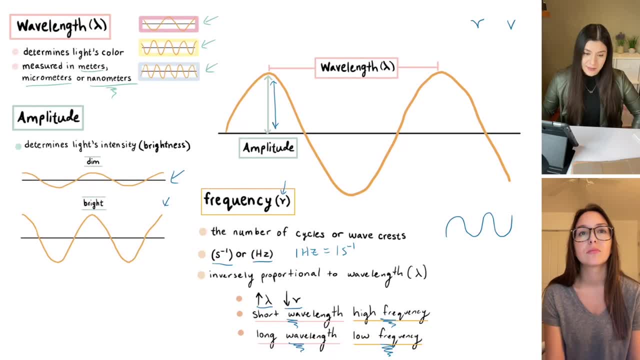 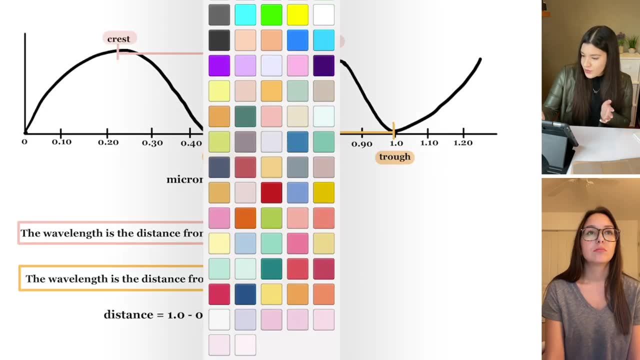 Okay, Any questions here? I don't think so. Okay, I know it's pretty straightforward for now. Yeah, Let's do a little bit more of the calculation side, but this is just looking at, uh, how to actually calculate a wavelength. 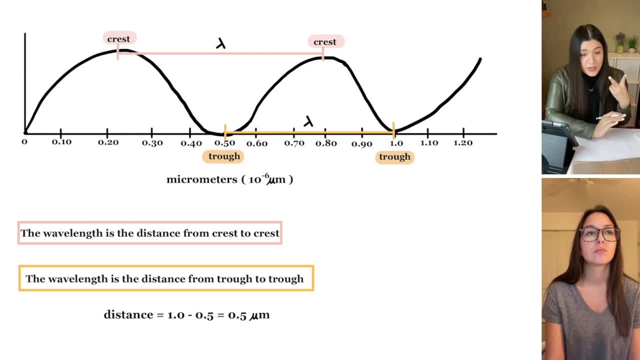 So if we were asked to calculate a wavelength, there's two different ways that we can do this. We can start off with just looking at the two different crests. So this, this would be this top part of our wave, would be our crest, This bottom part would be our trough. Okay, So those 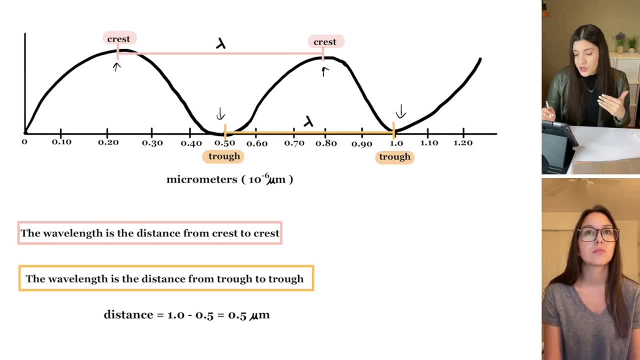 are just two different things: Top is crest, bottom is trough. And then if we were trying it, let's say if we were actually just given this number here, let's say this is, I don't know, 0.22, and then this was 0.78. 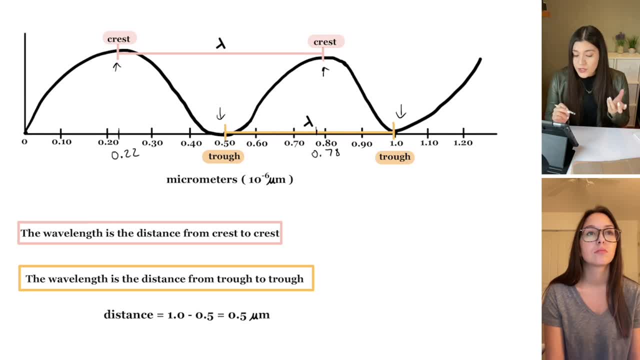 If we were only given those values, then what we would do to figure out the actual, uh like number for our wavelength is simply subtract. So larger number minus the smaller number, that would have been that 0.78 minus 0.22.. And then that would have been our wavelength. So in this case, uh, 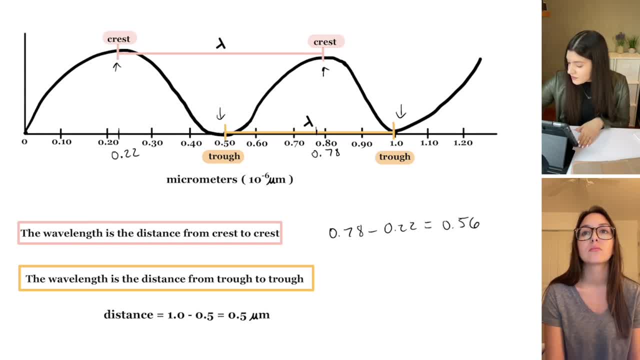 the actual subtraction is 0.56.. And then, whatever this is measured in, which is in micrometers, And then same thing goes, goes. if they were to just give us, like these actual values here for the trough, this is at one, this is at 0.5, we would simply subtract that distance and then we'd get the actual wavelength. 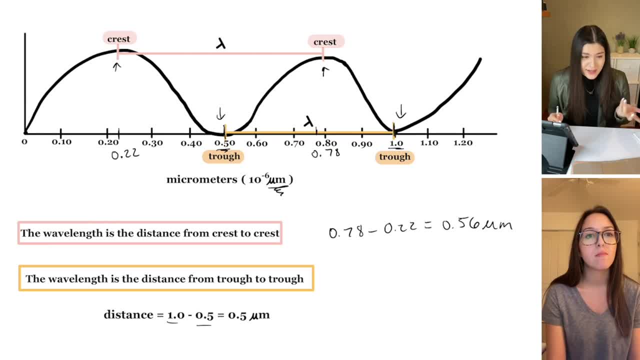 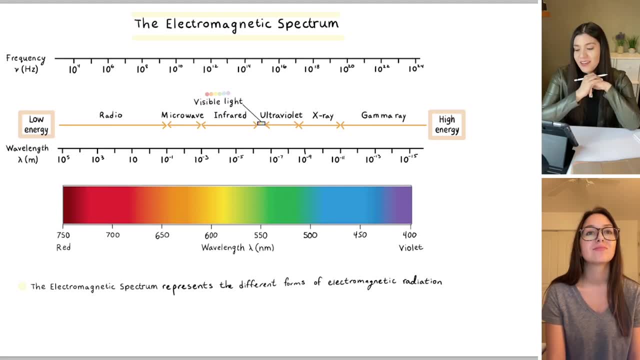 okay, so little simple things. that just in case you know. they have that on the multiple choice section. all right, the main main event here, so the electromagnetic spectrum. essentially what that does is it's just going to represent the different forms of the electromagnetic radiation or of light. right, so these are just different forms of light, essentially. so we would start off with i. 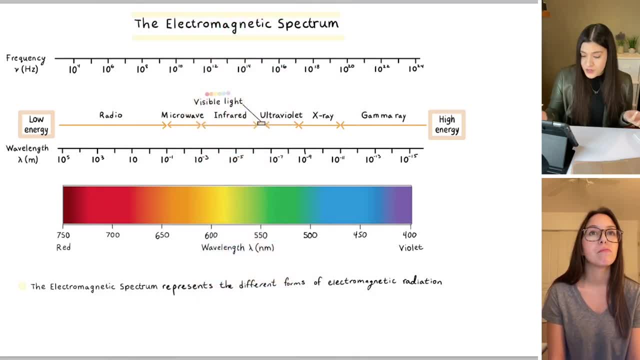 would say if you went over it. some professors do require you to know, kind of like, the different types of waves that you might see. that might be a factor. um, typically i haven't seen too much of that. it's more of the calculation side that they're really focused on. um, but 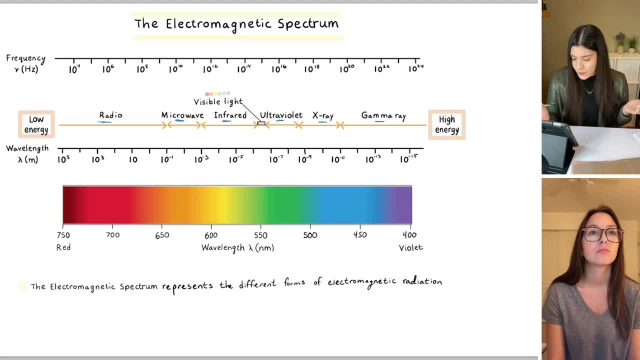 you. you, just in case he might be what we're going to find out in the practice exam either way. but um, one thing i want to also point out again is just seeing this relationship between the frequency and the wavelength. so as this starts to increase, our energy is then actually it's low here and then it's a little bit higher up there. 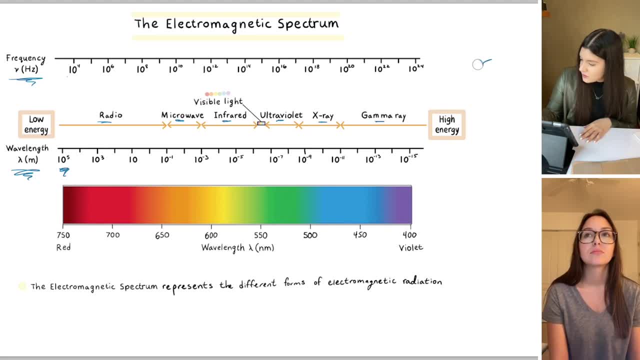 let me say that again. so our wavelength, we said as it goes up, the other goes down. okay, as we see that here, this is like 10 to the 5th. well, this is 10 to the negative 15th, which is smaller, and then this is larger. so the opposite. sorry, let me say this is larger. i know it's like 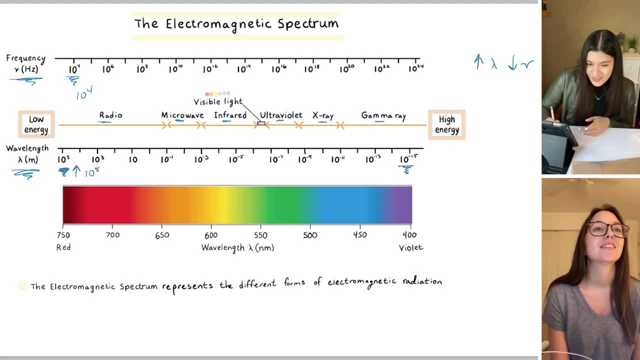 10 to the 5th- what's that? and then 10 to the 4th, okay, yeah. and then same thing here, like this is higher, right, this is at 10 to the 4th, and then 10 to the 5th, and then 10 to the 6th and then 10 to the. 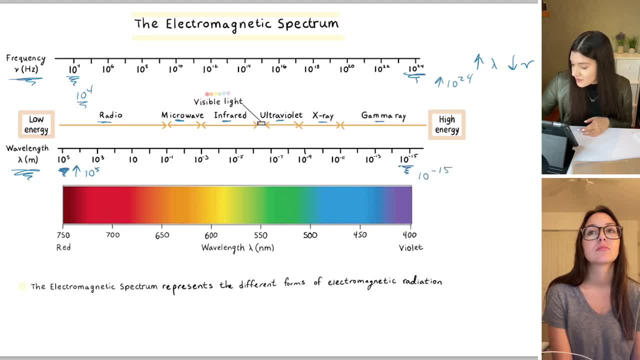 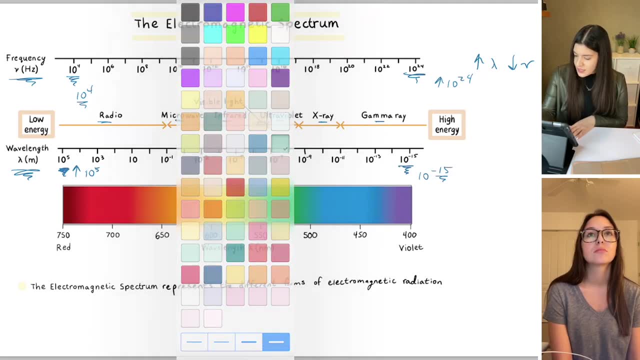 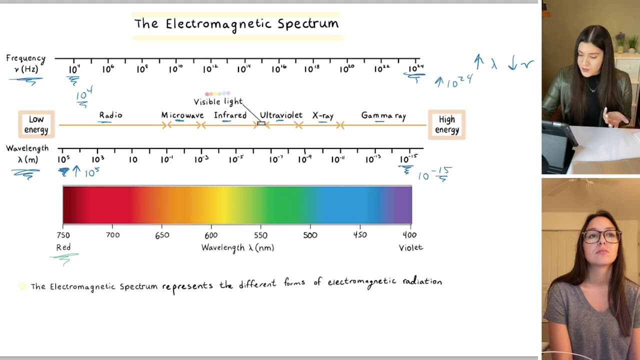 24th and then this is at 10 to the negative 15th, so negative exponent is going to be smaller. the other thing i will say to definitely know is at least understand that, like, oh, okay, the wavelength for, uh, visible light and, by the way, this is kind of like this right here, this little. 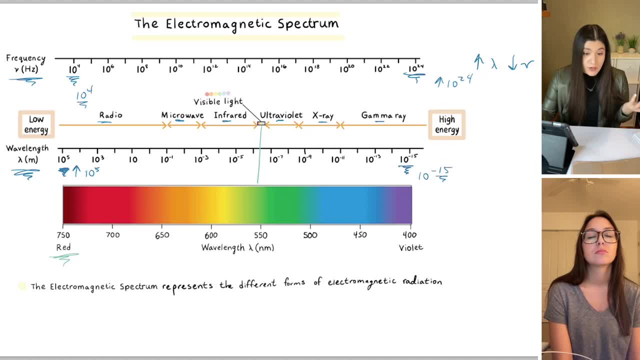 section, you're going to talk a lot about visible light, since that's what you know us as humans can see. um, we're going to see that like for, for a wavelength of like red, the color red that's going to be at 750. know that number, so know that range. the main ones that i typically see are either: 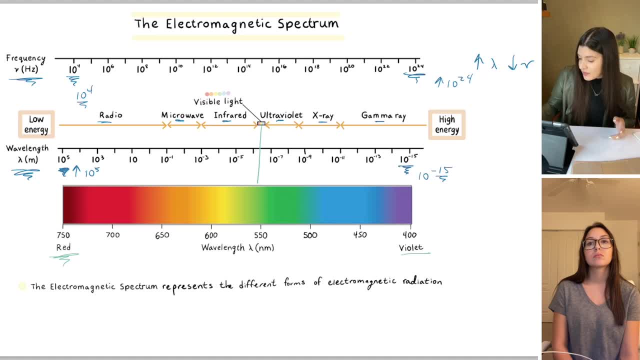 actually both different ends- is the red and then the purple, or violet in this case, which is 400 nanometers, because they may ask: oh, you know, what color is this. and then, like after you've you've solved for the wavelength, they may say: oh, what color is this? and then your wavelength is: i don't. 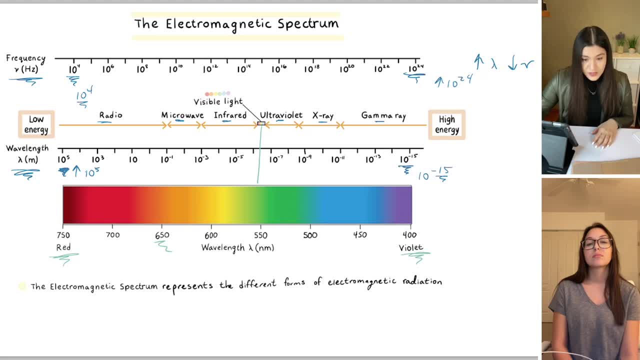 know 650. you know that's orange. oh, so i should know each of the colors and like about where they fall. about where they fall, yes, yeah, and the main ones i would say to like definitely know is like the ends- right, yeah, definitely the ends. definitely red. i see that one constantly, so that could be. 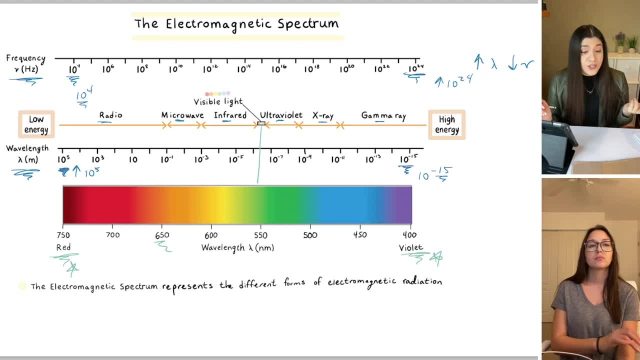 one thing. another thing is if they were to give you a bunch of wavelengths and tell you- and they would actually say, oh, arrange this, um according to increasing frequency, and then you would have to know the actual relationship between that and just knowing it's the opposite. so the 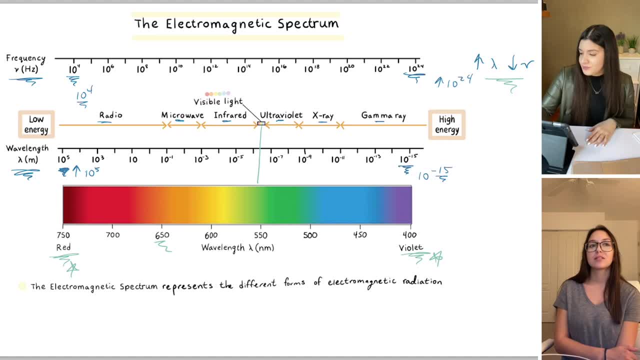 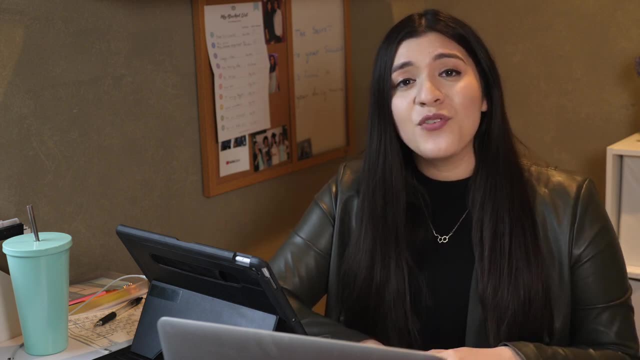 higher the wavelength, yeah, the lower the frequency- okay, so just little things that they may do for like. these are great multiple choice questions. okay. I hope you're learning a lot with this series, just like Melissa Lucia's. now, if you need additional help, then head on over to Melissa Maribel calm and I'll. see you in the next video.